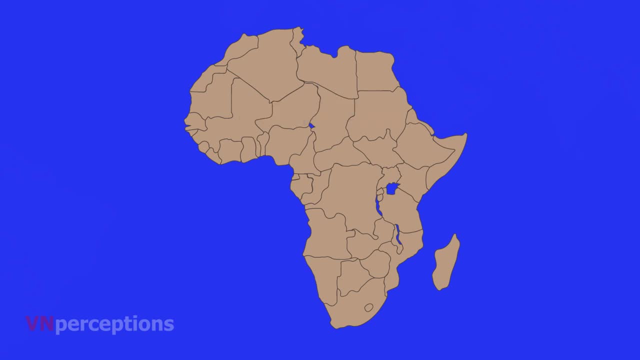 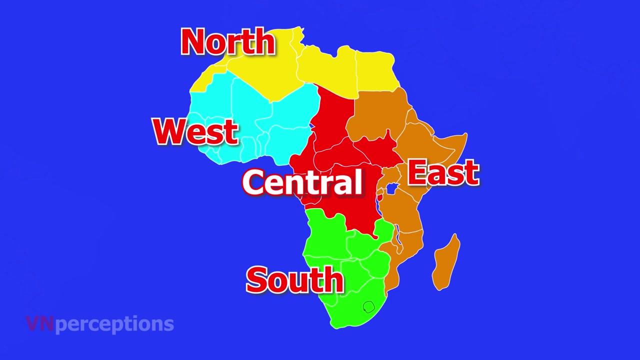 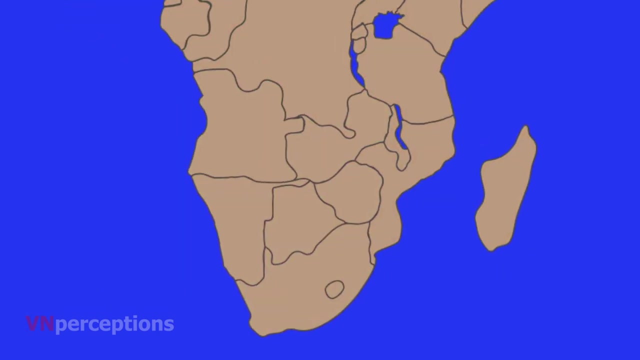 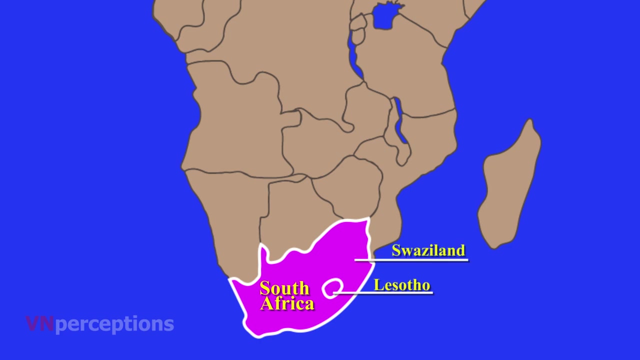 This entire continent is divided into five regions, ie North, South, East, West and the Central. Let us learn the names of the countries that lies within these five regions. The countries in the southern division are New Zealand, Namibia, Botswana, Zimbabwe, Mozambique, Malawi, Zambia and Angola. 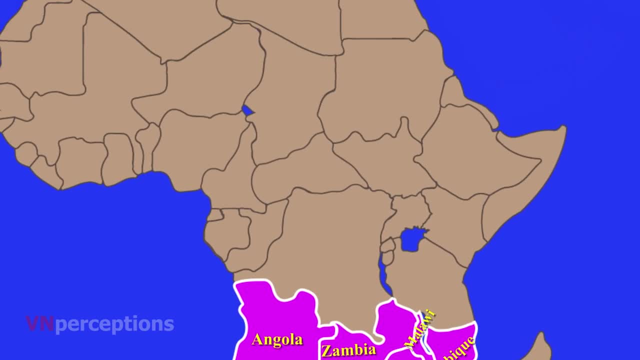 The countries of the central division are: Democratic Republic of Congo, Congo, Gabon, Central African Republic, Burundi, Cameroon, Chad, Equatorial Guinea, Sao Tome Principe. Then we come to the eastern division. Here the countries are: 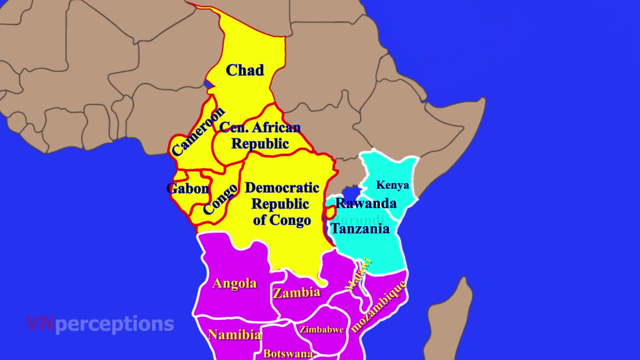 Tanzania, Rwanda, Kenya, Uganda, South Sudan, Sudan, South Sudan, Sudan, Kenya, Uganda, South Sudan, Ethiopia, Somalia, Eritrea, Djibouti, Madagascar, Comoros, Mauritius and Seychelles. 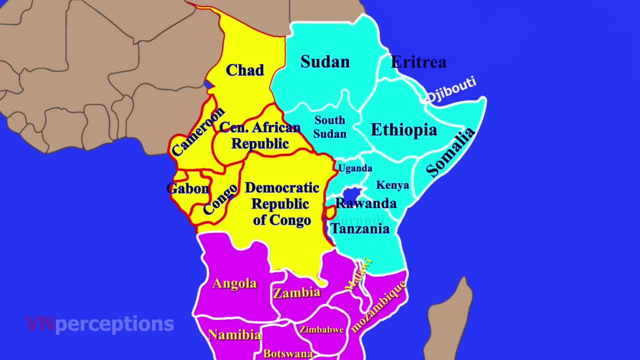 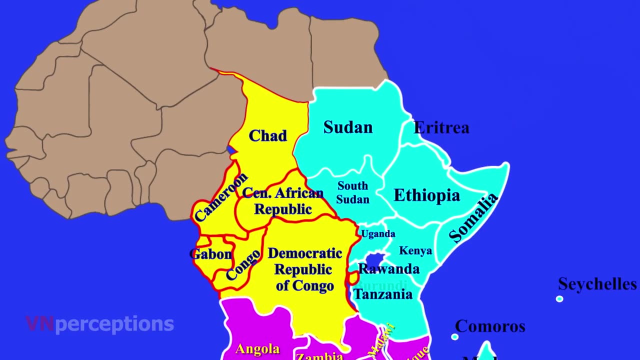 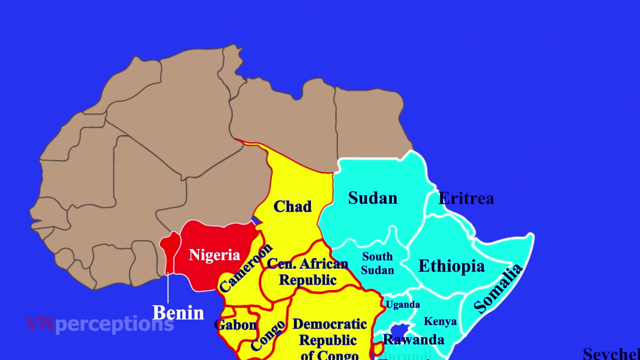 Ethiopia, Somalia, Eritrea, Djibouti, Madagascar, Comoros, Mauritius and Seychelles. In the western part, we have Niger Benin. In the western part, we have Togo, Ghana, Côte d'Ivoire, Liberia, Sierra Leone, Guinea, Guinea-Bissau, Gambia, Senegal, Mali, Niger, Burkina Faso. 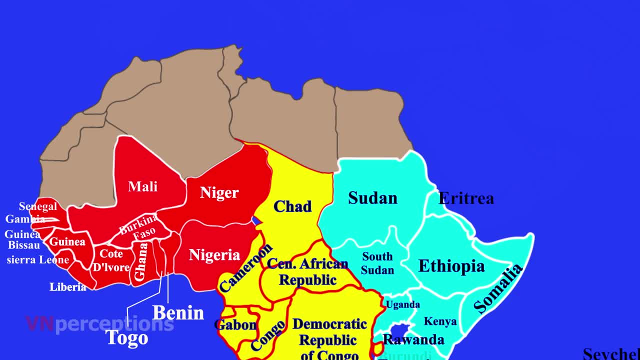 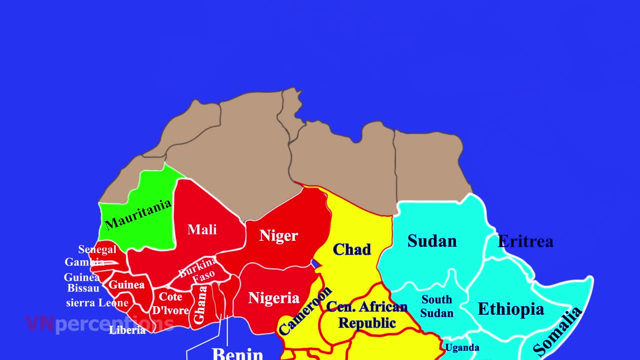 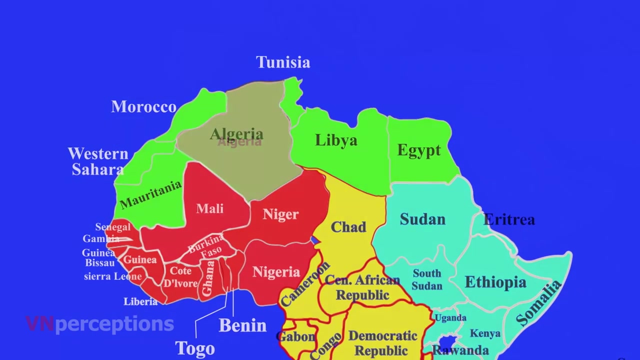 In the western part we have And Cape Verde. In the northern division we have Mauritania, Western Sahara, Morocco, Algeria, Tunisia, Libya and Egypt. Africa can be divided into many different regions. That is the desert region. That is the desert region. 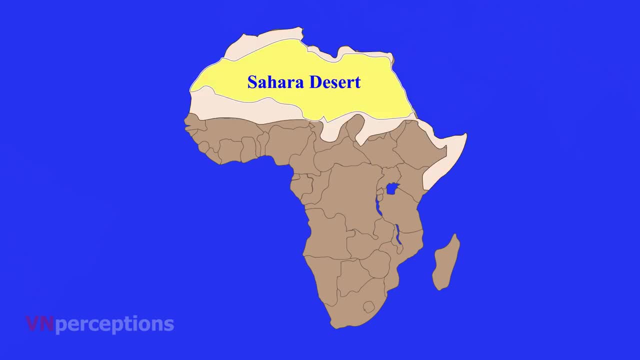 which includes the Sahara desert, Kalahari desert and the Namib desert. Then it is the tropical rainforest regions, Then savannah, Ethiopian highlands, Swahili coast and Southern Africa. Then the mountainous regions, like the Atlas mountain. 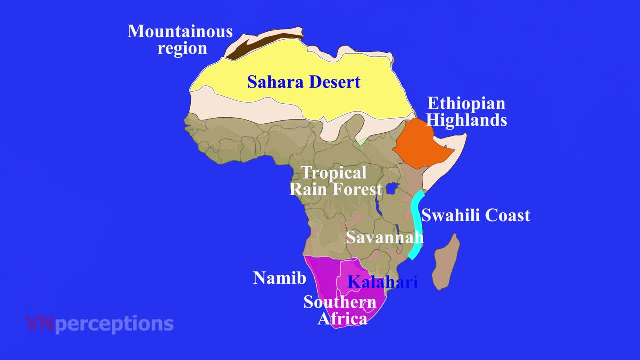 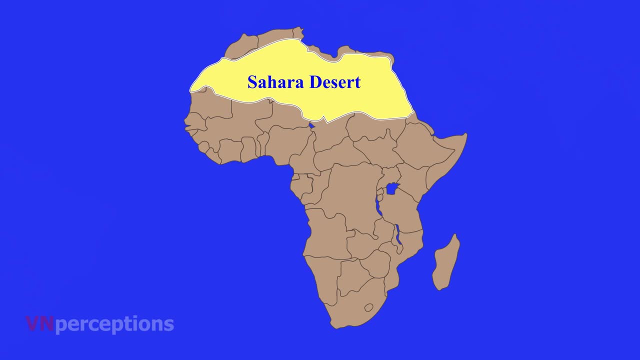 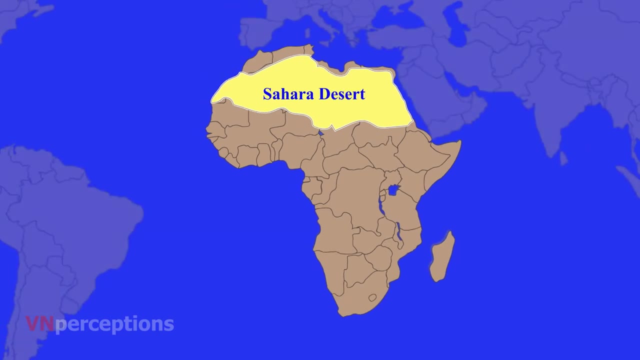 It is the largest hot desert in the world and third largest desert overall, after Antarctica and the Arctic. It has areas of 92 lakh square kilometers and is comparable to the areas of China and the United States. It has areas of 92 lakh square kilometers and is comparable to the areas of China and the United States. 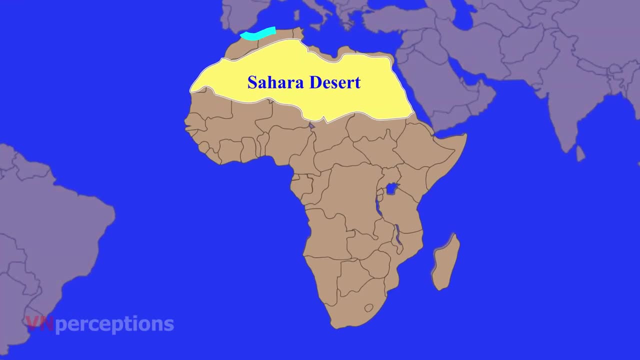 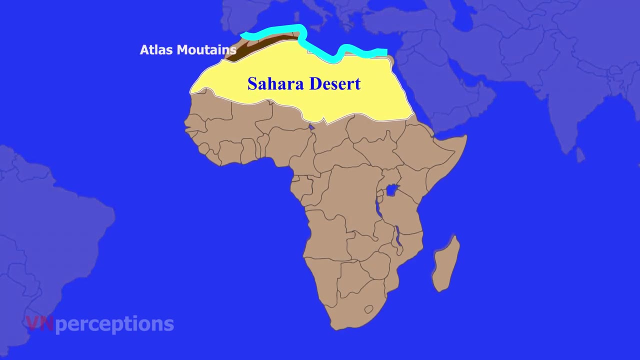 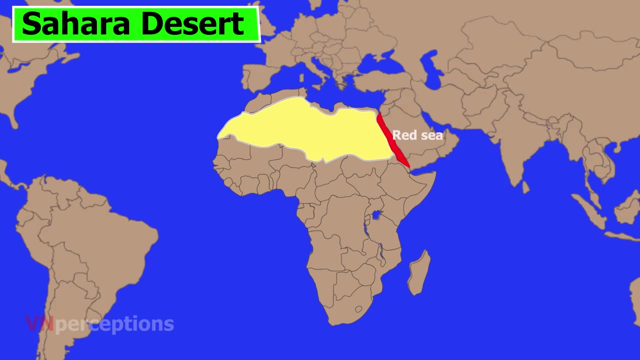 The desert comprises much of North Africa, excluding the fertile regions on the Mediterranean sea, Mediterranean sea coast, the Atlas Mountains of the Maghreb and the Nile Valley in Egypt and Sudan. It stretches from the Red Sea in the east and the Mediterranean in the north to the Atlantic Ocean. 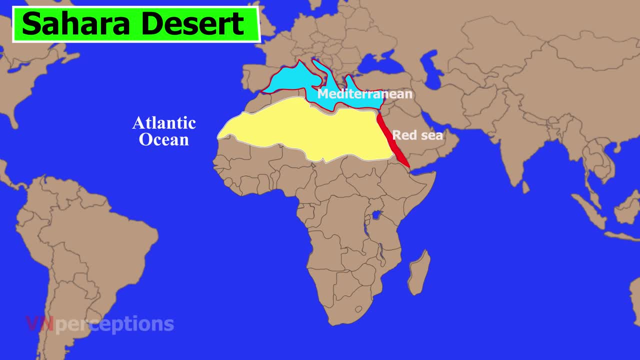 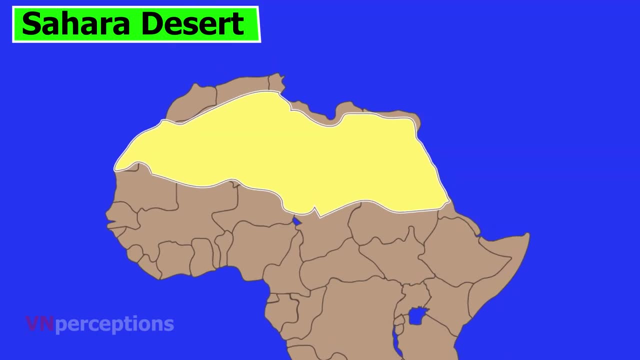 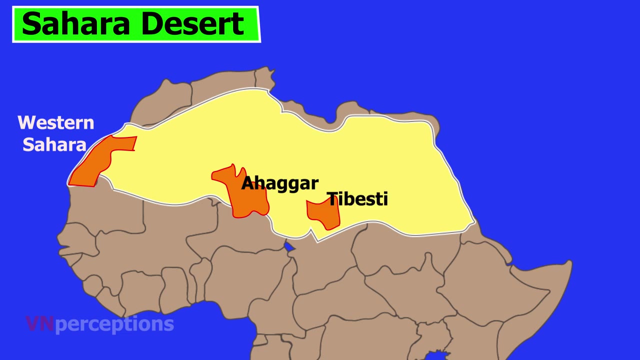 in the west, where the landscapes gradually changes from the desert to the coastal plains. The Sahara Desert can be divided into several regions, including the Western Sahara, the Central Aghar Mountains, the Tibesti Mountains, the Air Mountains, the Tenere Desert. 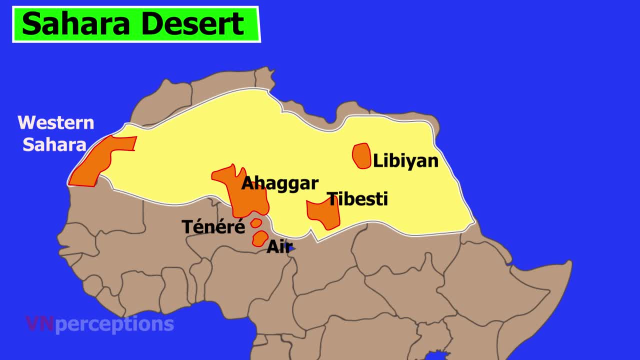 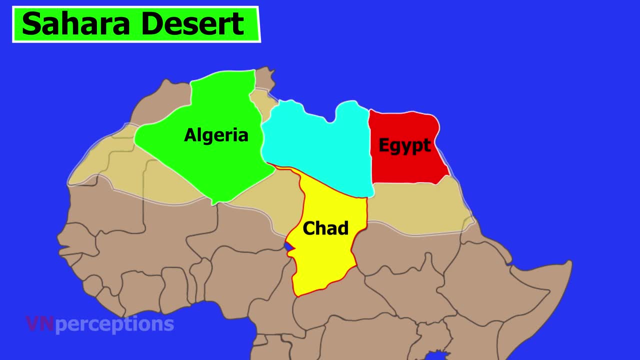 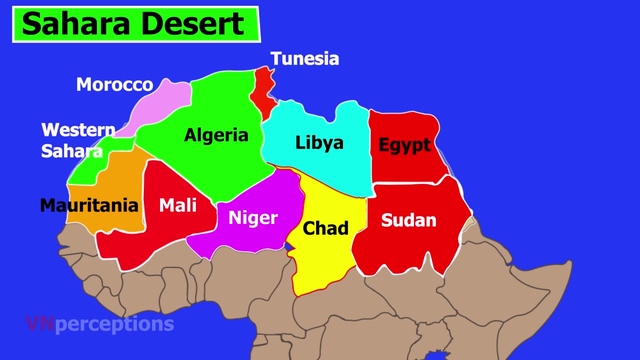 and the Libyan Desert and extends into 11 countries, And these are Algeria, Chad, Egypt, Libya, Mali, Mauritania, Morocco, Niger, Sudan, Tunisia, Western Sahara. The Sahara Desert is covered with sand dunes, rocky hills and stretches of gravel that continue. 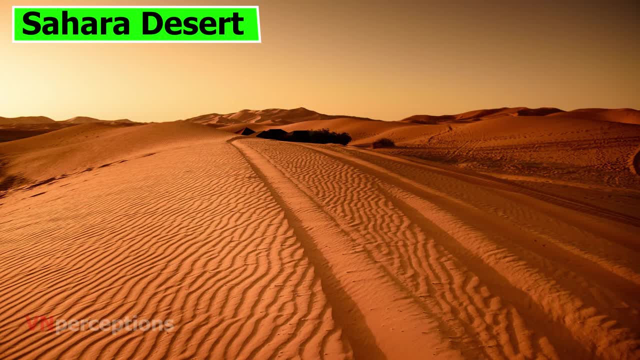 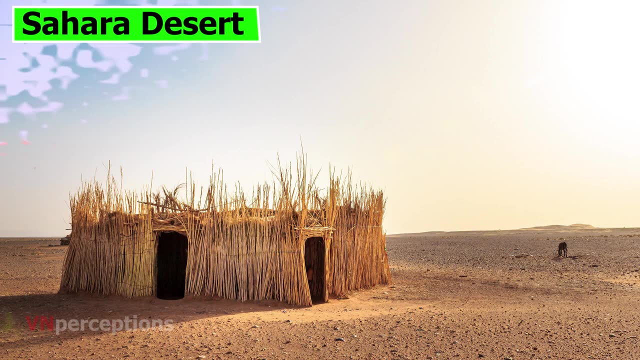 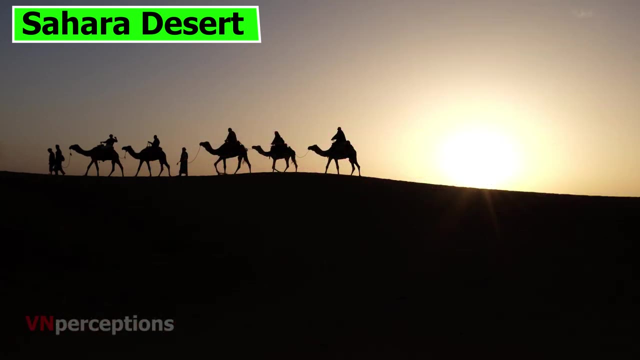 for miles and miles. Now very few people live in the desert, because it is considered one of the harshest places to live in the world. The people who live here are called nomads. They move from place to place, usually traveling by camel, looking for food and water. 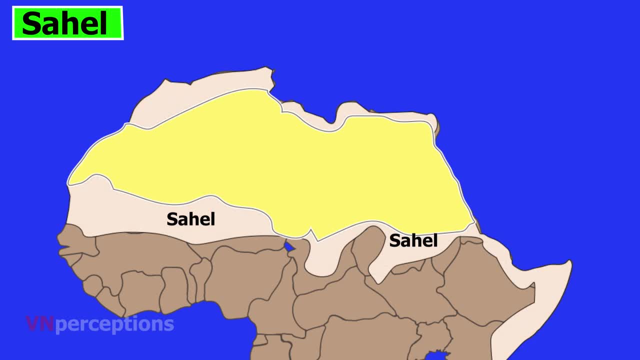 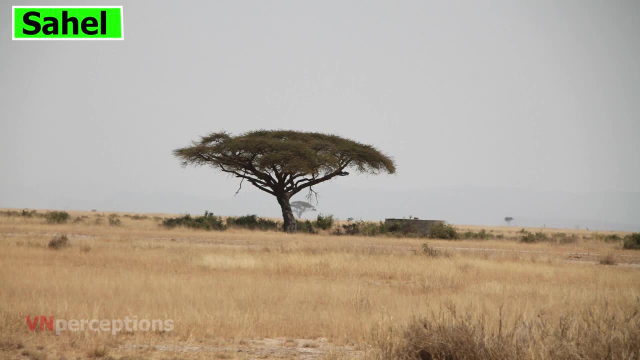 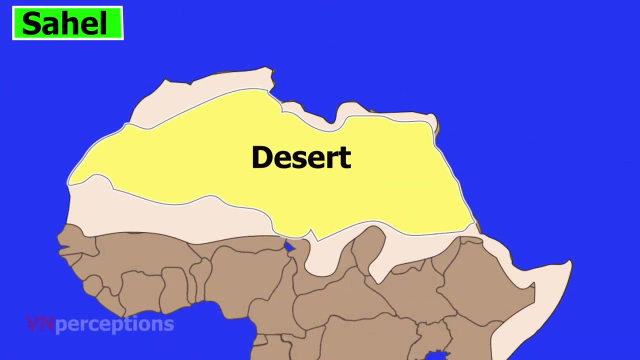 To the south is bounded by the Sahil. Talking about the Sahil, it is a strip of dry grassland that is located south of Sahara. The word Sahil means border or margin. It is a region between the desert to the north and the grasslands and rainforest to the south. It is a dry, semi-arid. 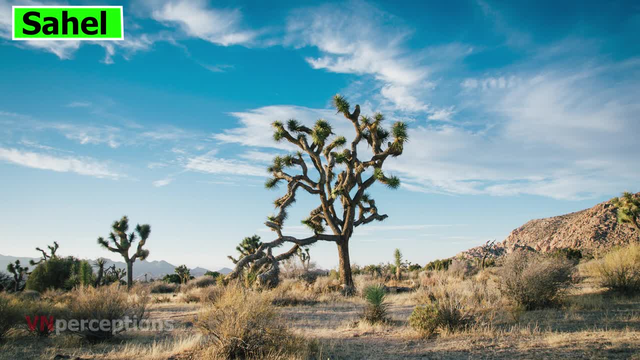 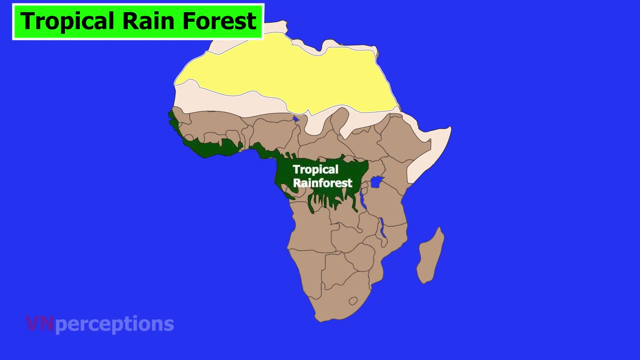 region that is slowly turning into a desert. It gets more rainfall than the desert, but still receives very little, ranging from 6 to 20 inches. We go to the next division, and that is the Africa's tropical rainforest. Now it is located along the central coast. 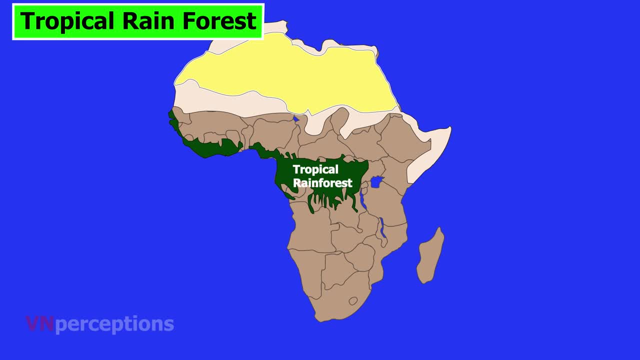 of Africa near the equator, It mainly lies in the Congo River Basin. The rainforest covers one-fifth of the land surface of Africa and touches 37 countries. It is the second largest rainforest in the world and the Amazon. The Amazon rainforest in Brazil is the largest. The rainforest has a hot and humid climate. 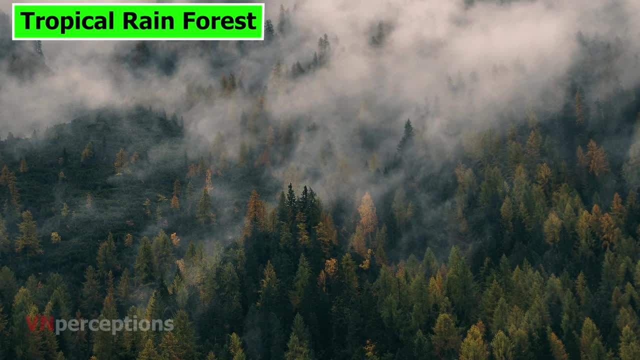 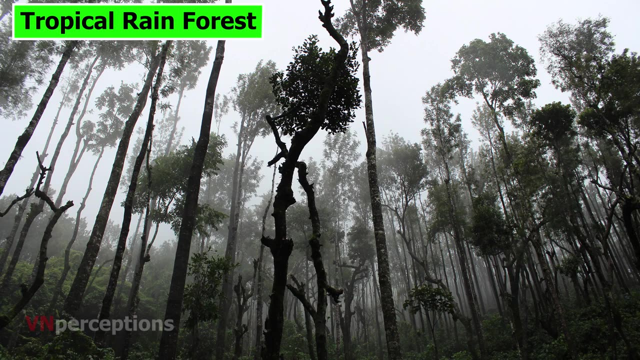 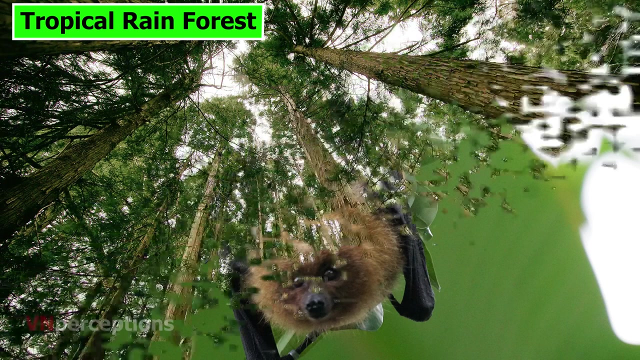 It rains for about 117 days per year, with a total of approximately 1766 millimeter of rainfall. There is a large variety of animals found in this region. The trees are also so thick and tall that sunlight never reaches the forests floor. The trees grow hundreds. 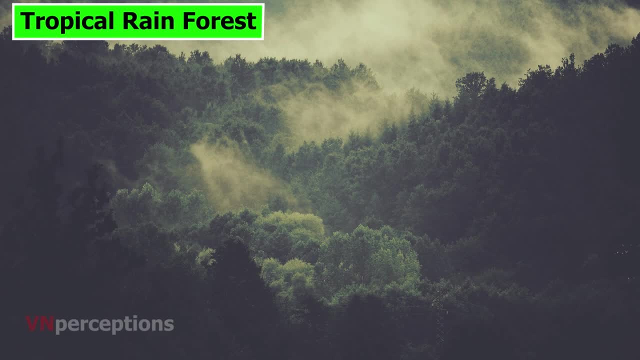 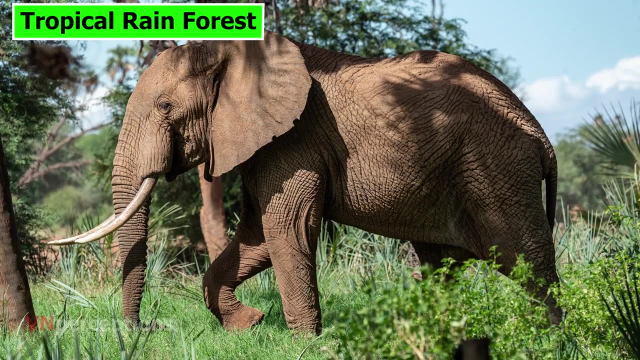 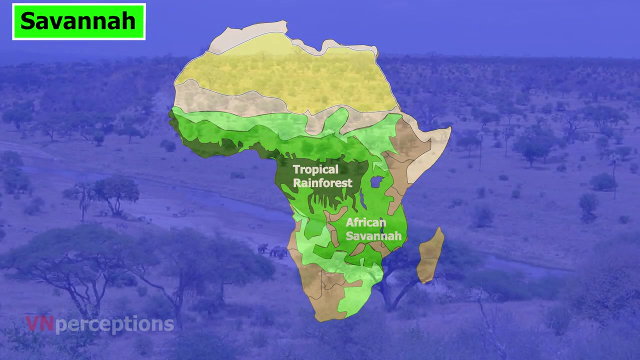 of feet high. all the Congo rainforest is famous for its gorillas, chimpanzee and elephants, as well as its native population of forest dwellers known as pygmies. Now we come to African savannas. The savannas are areas of open grasslands with dispersed trees, grasses and tall and thick. 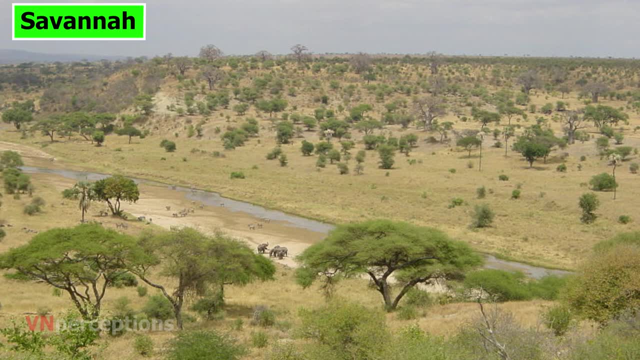 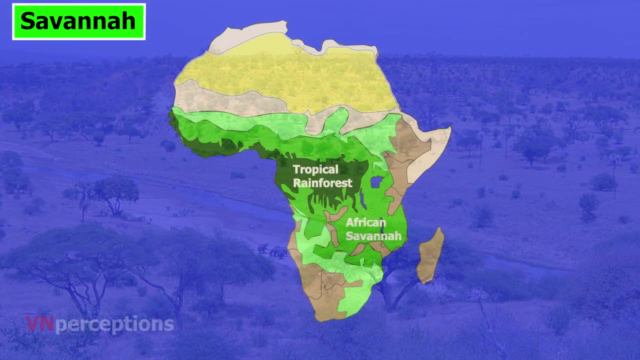 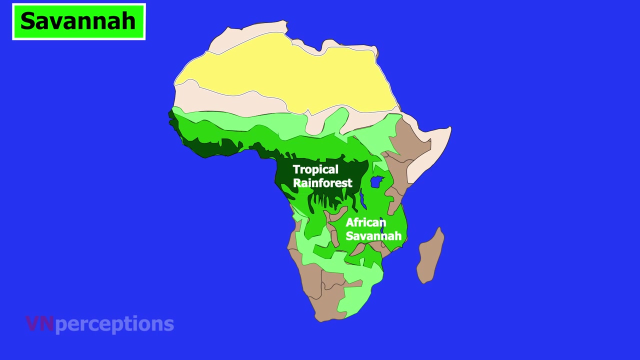 while trees are short and scattered. Well, African savannas are hot, dry grasslands that are located near the equator and cover almost half of Africa. They actually cover the region just north and south of rainforest that lie along the equator. The African savanna is the largest in the world. 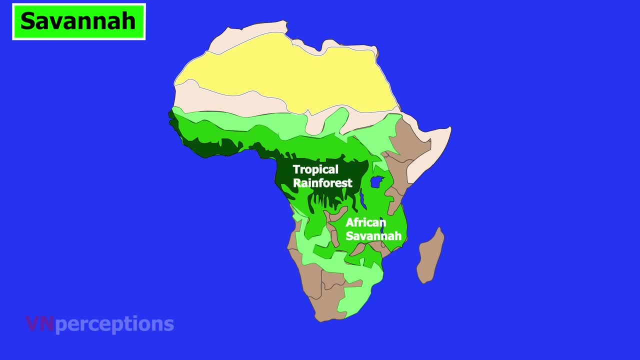 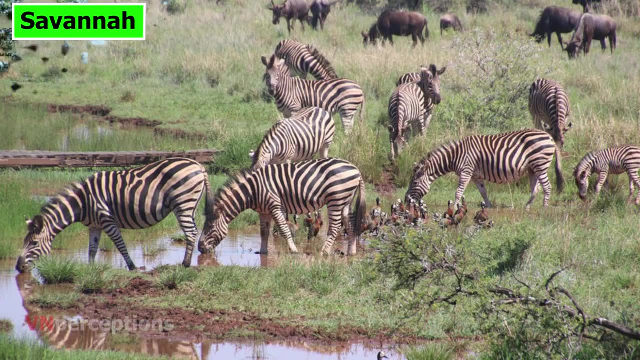 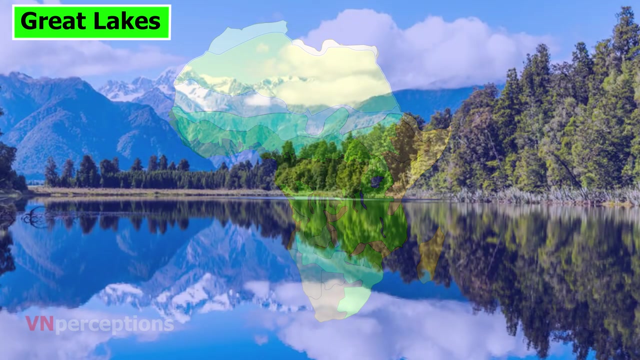 Nearly half of the continent of Africa is covered with savanna grasslands. There is a large variety of wildlife here, including lions, zebras and elephants. Then comes the African Great Lakes. Well, it is a system of natural water features that flow in the valley. Together they comprise some 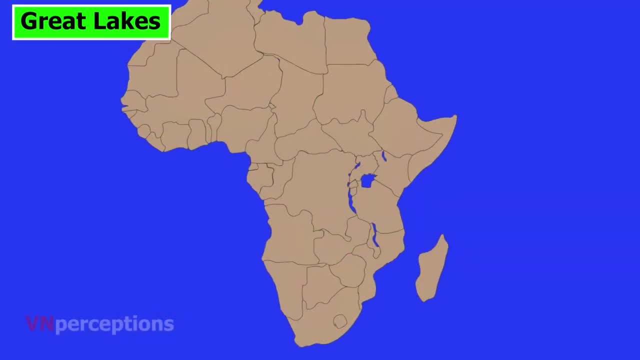 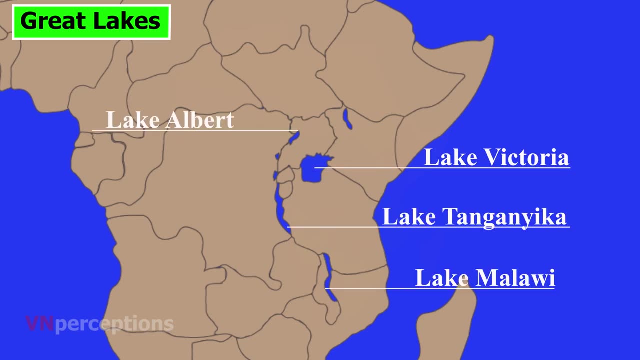 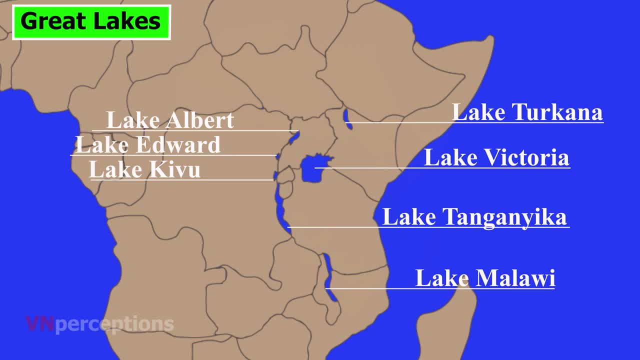 Turkana. Together, they form the seven major African Great Lakes. Lake Tanganyika is located in Central Africa. It is divided between the Burundi, Congo, Tanzania and Zambia. Lake Tanganyika is the deepest lake in Africa and one of the deepest in the world. It is also one of the 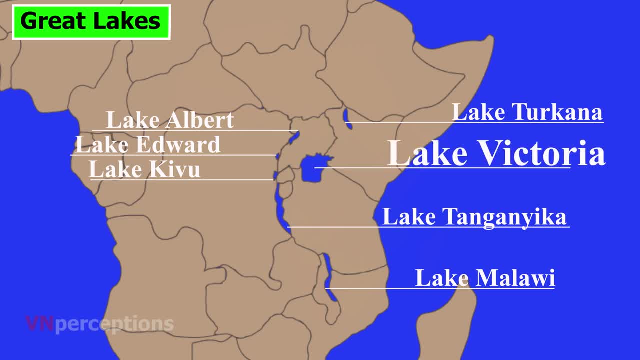 largest freshwater lakes in the world. Lake Victoria is the largest freshwater lake in the world. Lake Victoria is the largest freshwater lake in the world. Lake Superior is the largest. It is located in Central Africa and extends into three countries, ie Tanzania, Uganda and Kenya. While 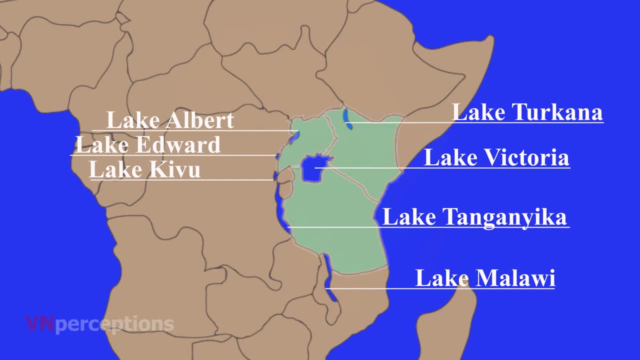 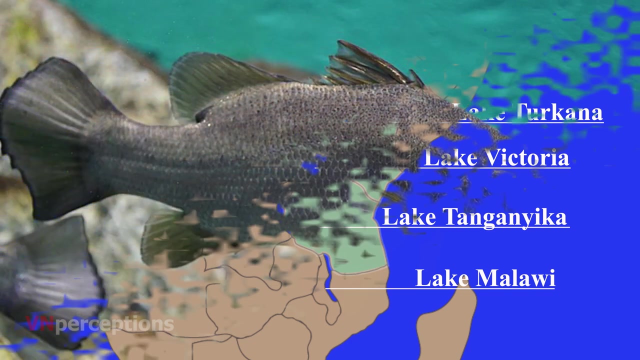 Nile begins here. Lake Victoria is vital in supporting the millions of people that live nearby. It provides a living for many fishermen and attracts millions of tourists each year. This region has a large reserve of aquatic and terrestrial life forms, Most of them usually living near the surface or deep under the water. These include the Nile perch fish wild beast. 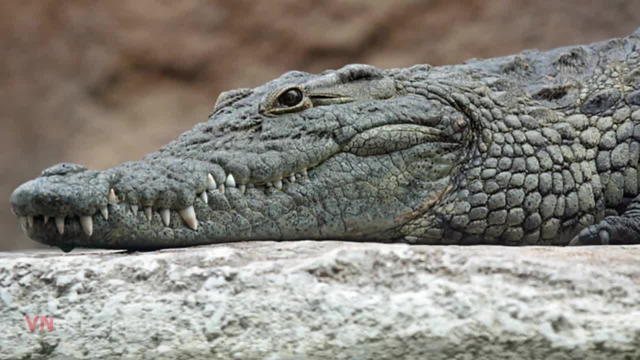 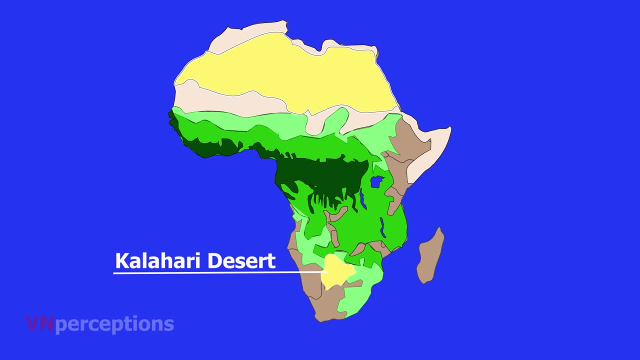 hippos and crocodiles. Then we come to Kalahari Desert. Kalahari Desert is located in the southwestern Africa. It covers parts of Botswana, Namibia and South Africa. The region is located in the north-east of Ethiopia. It is surrounded by semi-arid areas that are slowly becoming more dry. 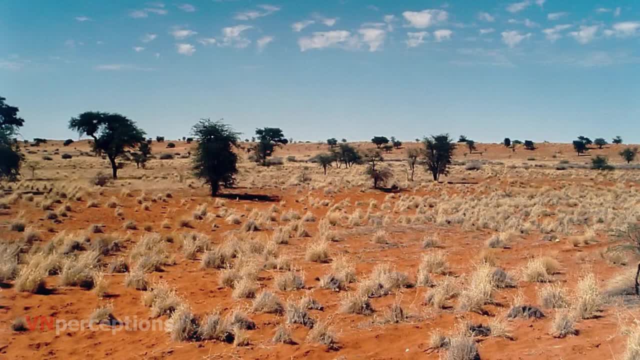 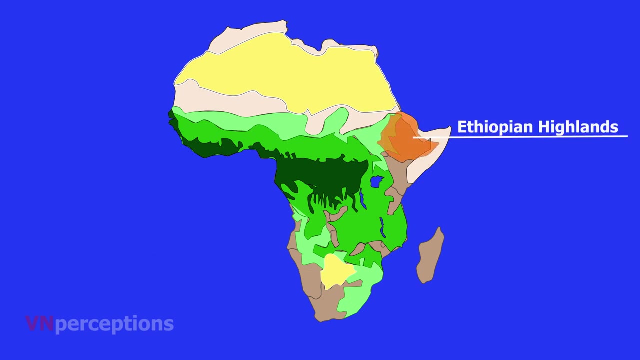 It is not a true desert because it receives 3 to 10 inches of rain per year. Because of the precipitation and underground supplies, grass, shrubs and wild animals manage to live in the Kalahari desert. Then we come to Ethiopian Highlands. Ethiopian Highlands is a rugged mass of mountains in Ethiopia, situated in the Horn, Riyadh and 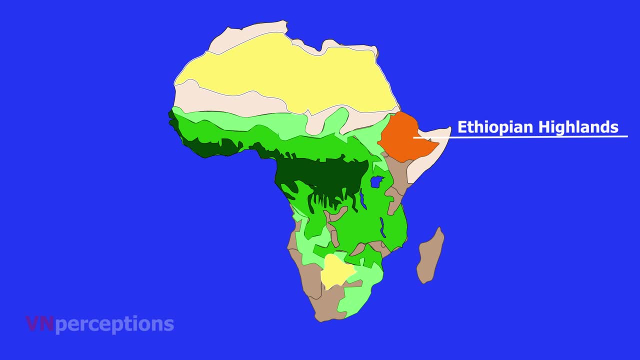 Sintra region in north-east Africa. It forms the largest continuous area of its elevation in the continent, with little of its surface falling below 1,500 m, while the summits reach a height of 4,550 m. It is sometimes called the roof of Africa due to its height and large area. Most of the Ethiopian Highlands are part of Central and North Ethiopia and its northernmost portion of the North African region. 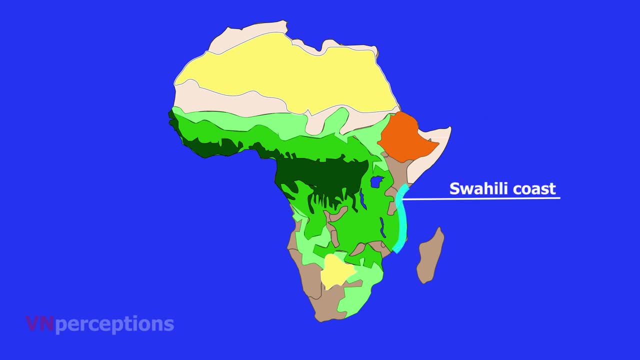 reaches into Eritrea. Then we come to Swahili coast. The Swahili coast makes up one of the geographic region of Africa with the least number of wildlife. The stretch consists of the coastline extending from Somalia to Mozambique. The Swahili coast consists of sandy beaches and maritime plant. 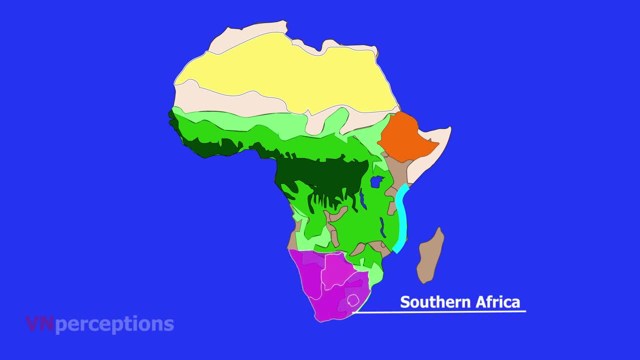 life. Then we come to Southern Africa. This should not be confused with South Africa. Now, this is another great reserve of wildlife among the geographic regions of Africa. Southern Africa has a shelf of bedrock known as the Kapawal, extending throughout. The area is rich in. 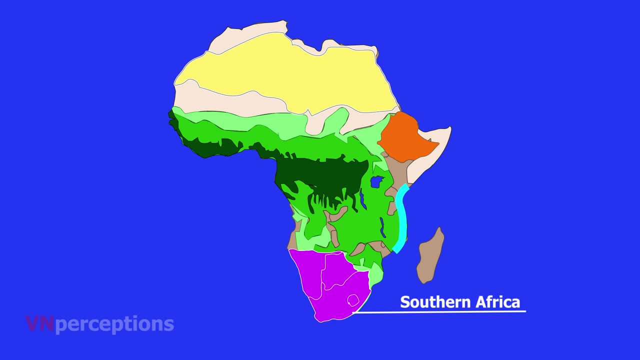 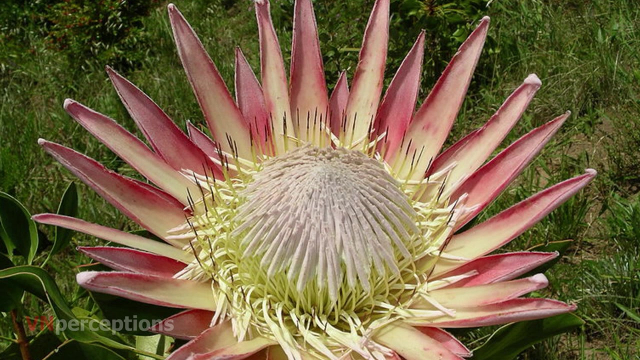 mountains and plateaus. The region has some of the Africa's richest plant species varieties, and some are native to the region. These include the giant Protia, which happens to be South Africa's national flower. This species thrives in the Cape Flora area. There is also a plenty of animal species that find. 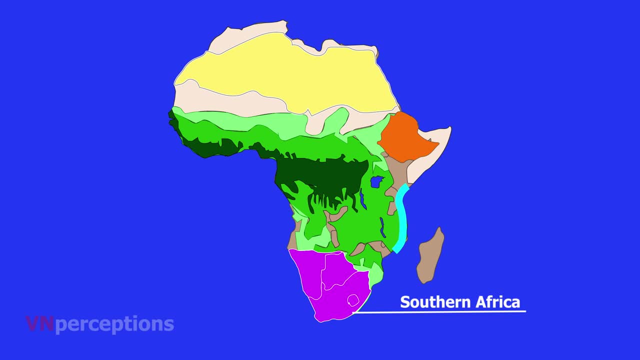 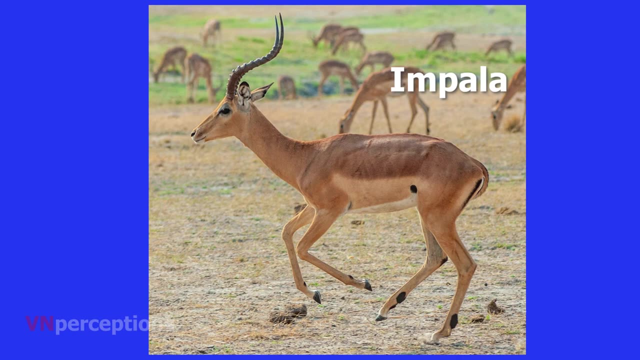 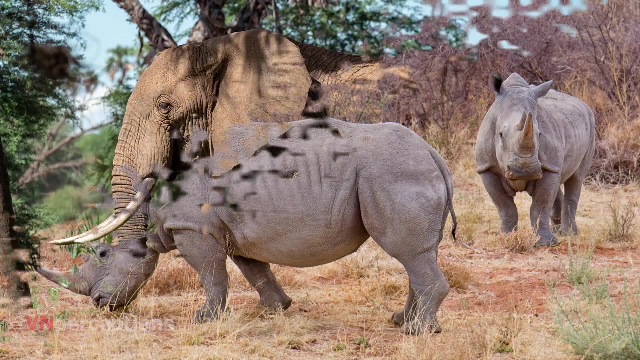 refuge in this lush wildlife. They include the graceful Impala and a menacing Big Five famous for their hard-to-hunt reputation, ie the Lion, Leopard, Rhinoceros, Elephant, Cape Buffalo Baboons and Burschel Zebras. 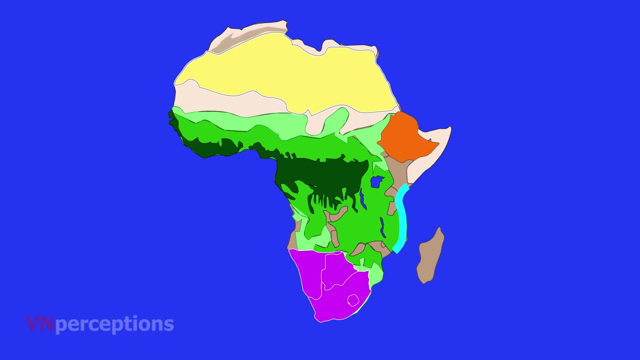 Also call this place home. Then comes the Atlas Mountains. Well, Atlas Mountains are the mountain ranges in North Africa. The mountains extend from Morocco to Tunisia, between the Mediterranean and Sahara Desert. They separate the coastal region from the Sahara Desert. Then comes the Eastern. 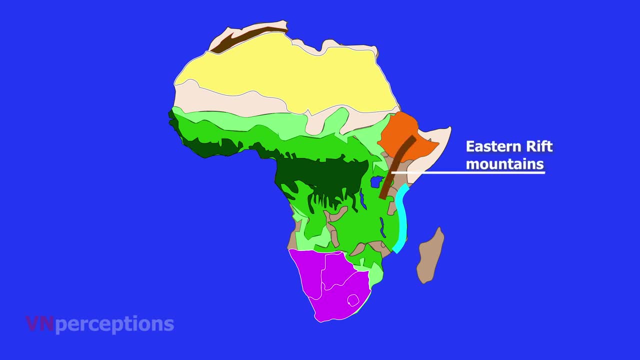 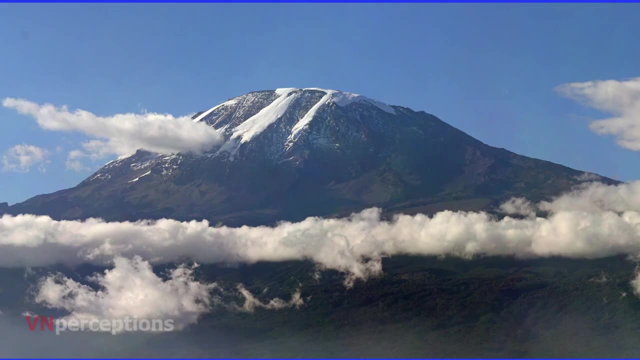 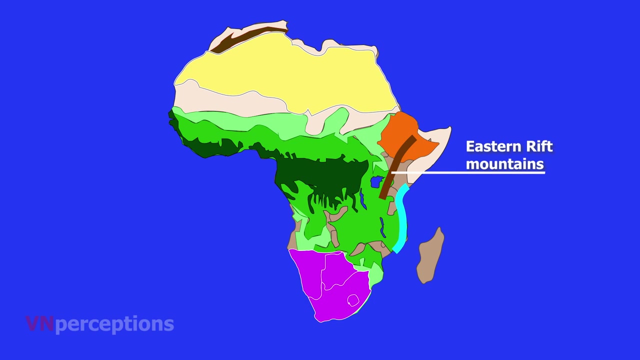 Rift Mountains, which has the famous mountain, ie the Sahara Desert. The Sahara Desert is a mountain that extends from Jordan in southwest Asia southward through eastern Africa to Mozambique, And this is totally 6400 kilometers long and averages 48 to 64 kilometers wide. It has 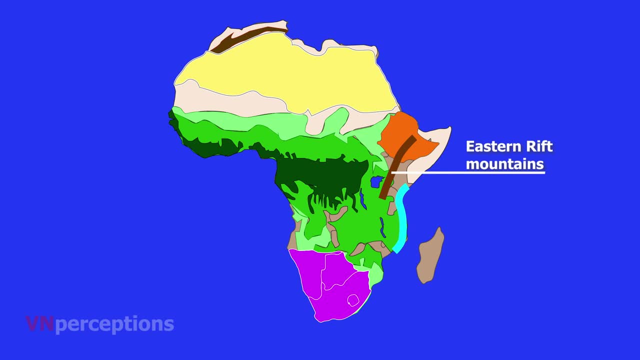 Mount Kilimanjaro and Mount Kenya. Then it is Drakensberg Mountains. The Drakensberg Mountains are the mountain ranges in North Africa. The mountains extend from Morocco to Tunisia, between the Mediterranean and Sahara Desert. The Drakensberg Mountains is the name given to the eastern portion of the Great Escarpment which encloses the central. 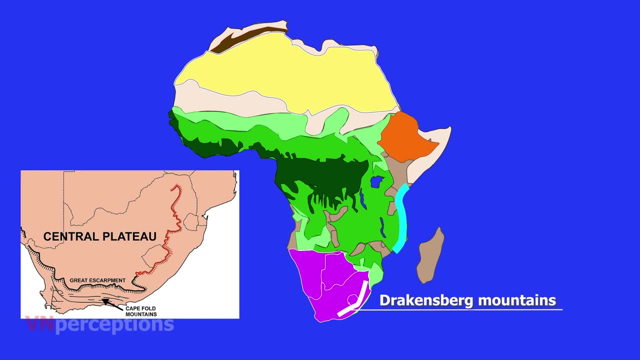 southern African plateau. The Great Escarpment reaches its greatest elevation in this region, ie 2000 to 3482 meters. It is located in South Africa and Lesotho. Thank you for watching.